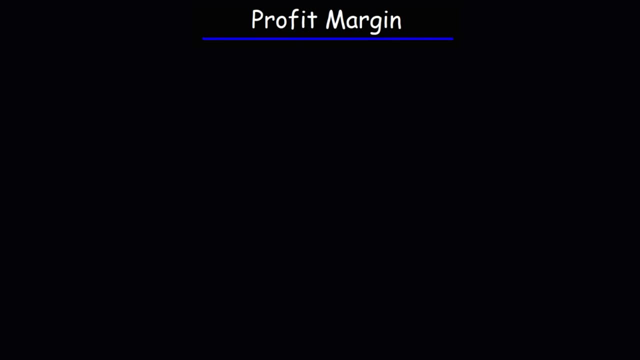 In this video we're going to talk about the profit margin, the gross margin and the operating margin. So let's talk about the profit margin, also referred to as the net profit margin. So this value is equal to the net income divided by the annual sales of the company, or the sales for the last 12 months, times 100%. 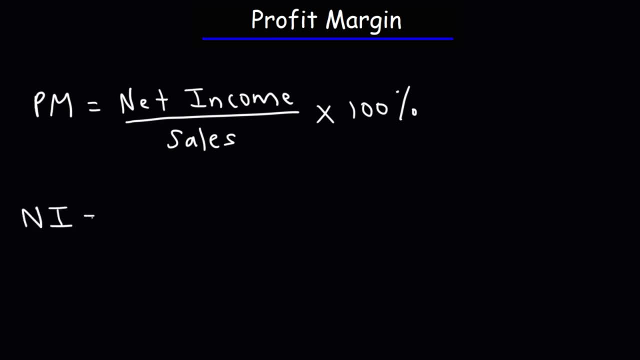 Now keep in mind: the net income is the difference between the sales, which is the same thing as the revenue, minus all of the expenses. So I'm going to write TE for total expenses. So let's look at an example. 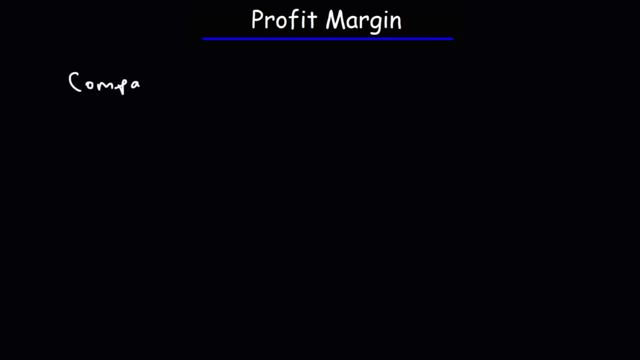 So let's analyze two companies. Let's just call this Company A and Company B. So let's say that Company A had sales of $100 million, just to use nice numbers, and Company B had the same annual sales of $100 million. 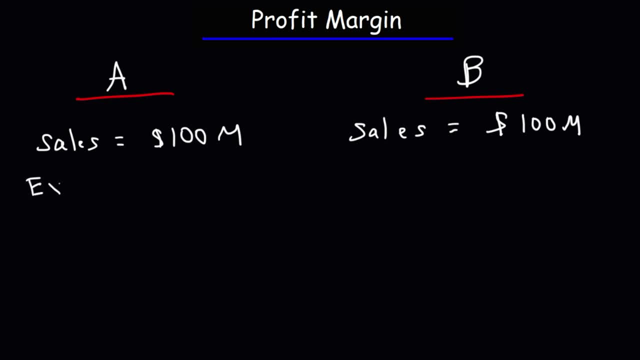 Now the total expenses for Company A, let's say it's $80 million, Whereas the total expenses for Company B for that year, we're going to say it's $50 million. So which company has the larger profit margin? 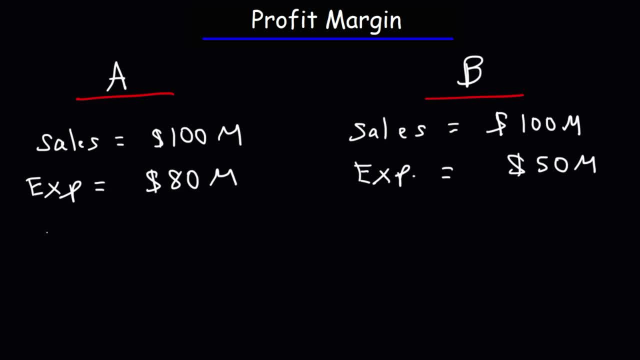 Would you say it's Company A or B? Well, first we need to calculate the net income for each company. So the net income is the difference between the sales and the total expenses. So $100 minus $80, that's going to be $20 million in net income for Company A. 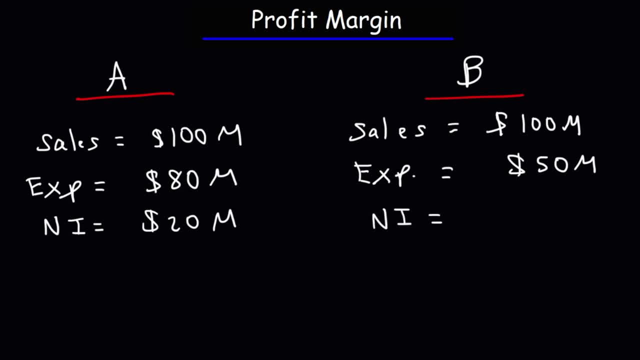 For Company B, the net income is going to be $100 minus $50.. So it's going to be $50 million. Now the profit margin for Company A is going to be the net income divided by the sales. So you have $20 million divided by $100 million times 100%. 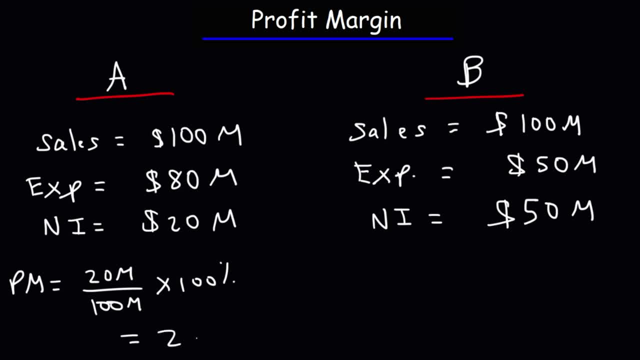 So Company A is going to have a profit margin of 20%. So what this means is that 20% of the sales were generated as net income. Now let's calculate the profit margin for company B. So company B had $50 million in net income and the annual sales is $100 million. 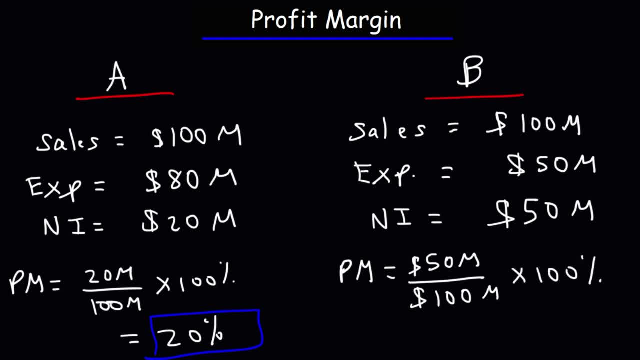 We're going to multiply that by 100%. So 50 divided by 100 is 0.5.. 0.5 times 100%, That's equal to 50%. So company B has a profit margin of 50%. So this tells us that 50% of the sales were net income. 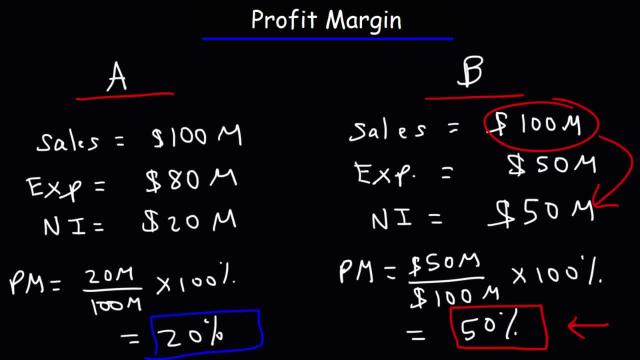 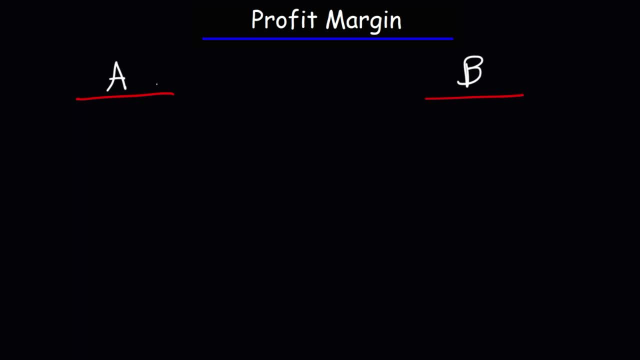 So 50% of 100 is 50.. Now let's look at this from another perspective. So let's say company A, Okay, Had sales or revenue of- let's use $1 billion. Now let's say company B had the same. actually let's use the same number. 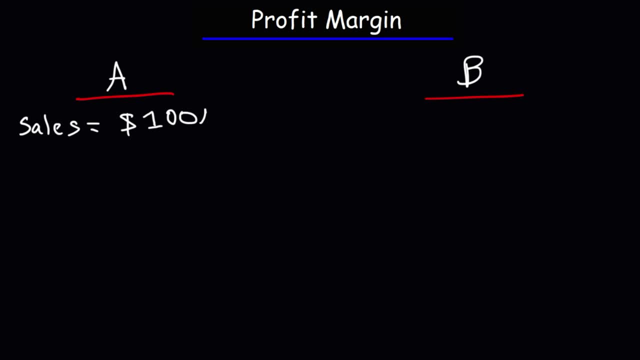 Let's use $100 million- 100 is a nice number- And we're going to say that company B had the same sales just like before, But this time I'm going to give you the profit margin. So let's say that company A has a profit margin of 30%. 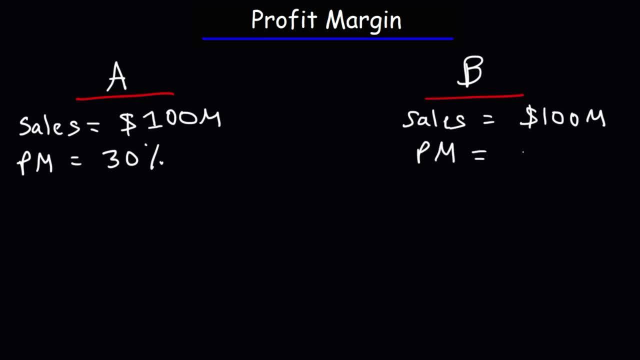 Whereas company B has a profit margin of, let's say, 20%. What is the net income for each of these two companies? To calculate the net income, it's simply the sales multiplied by the profit margin, divided by 100. So the profit margin is 30%. 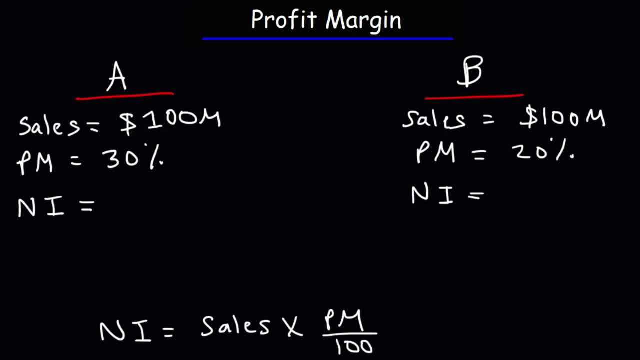 As a decimal, that's 0.30.. So 30 divided by 100 is 0.30.. So really, to find the net income, you just got to find out what 30% of 100 is. 30% of 100 is 30.. 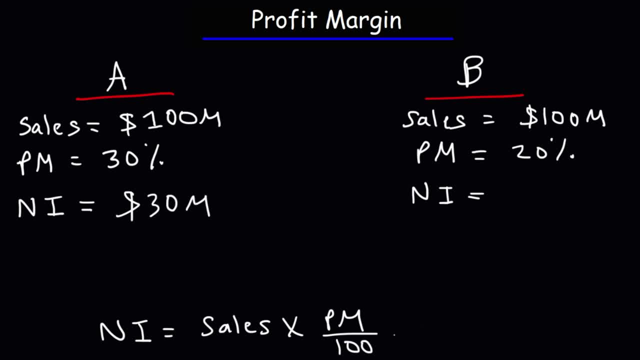 So the net income for company A is 30 million. Using this formula, it would be 100 million times 30% divided by 100. So these will cancel, You'll just get 30.. Now company B has the same annual sales but a profit margin of 20%. 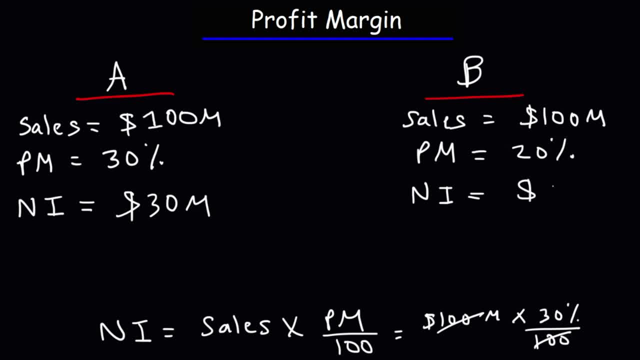 20% of 100 million is 20 million, And so if you know the annual sales of the company and you know the profit margin, this can give you a good idea of the net income that this company is making. Now let's go back to the formula that we had before. 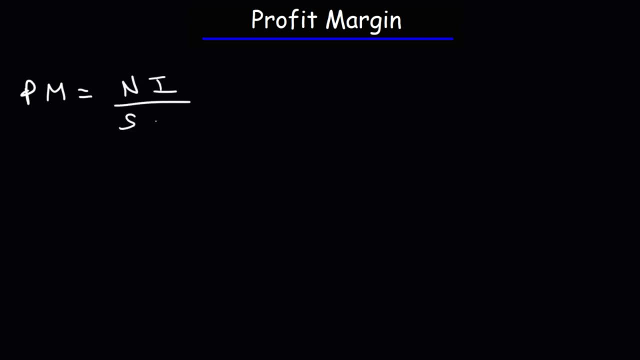 So we said that the profit margin is the net income divided by the sales Times, 100%, And the net income is basically the sales or the revenue minus the expenses over the sales, which is the same as the revenue. So as we increase the revenue, what happens to the profit margin? 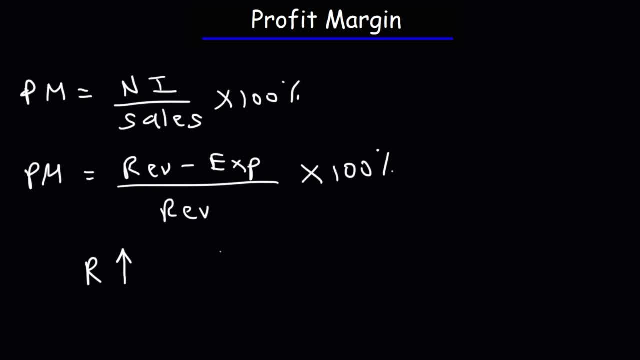 Will it increase or decrease? As the revenue increases and if the expenses are held constant, the profit margin will decrease. margin increases As the expenses increases, the profit margin decreases. So you have two ways in which you can increase the profit margin: Increase the revenue or decrease the expenses. So that's. 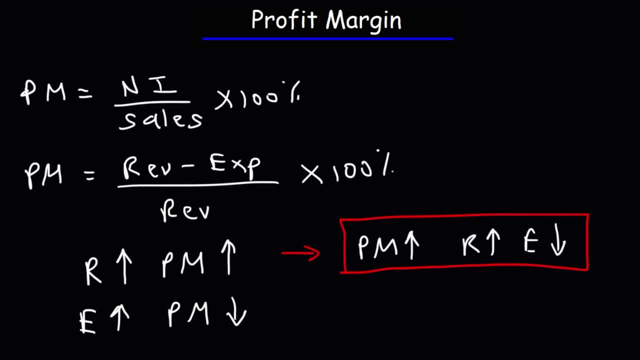 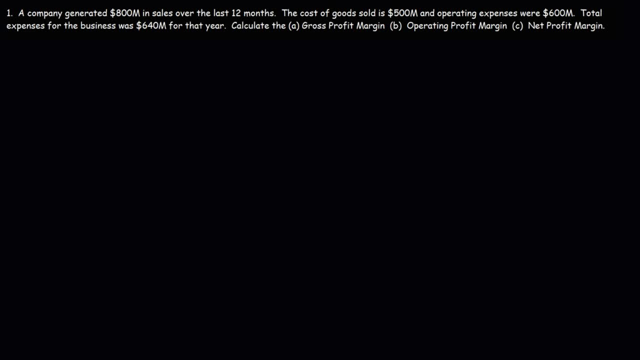 another concept that you need to understand, which is pretty intuitive, but it's good to have that down in your notes. Let's work on this problem. A company generated 800 million in sales over the last 12 months. The cost of goods sold is 500 million and operating expenses were 600 million. 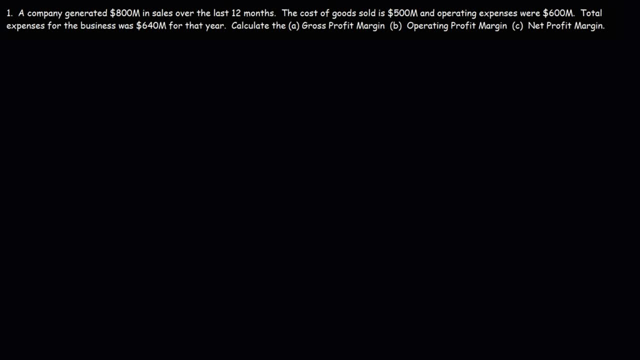 Total expenses for the business was 640 million for that year. Calculate the gross profit margin, the operating profit margin and the net profit margin. So let's start with the gross profit margin, which I'm going to abbreviate as GM gross margin. 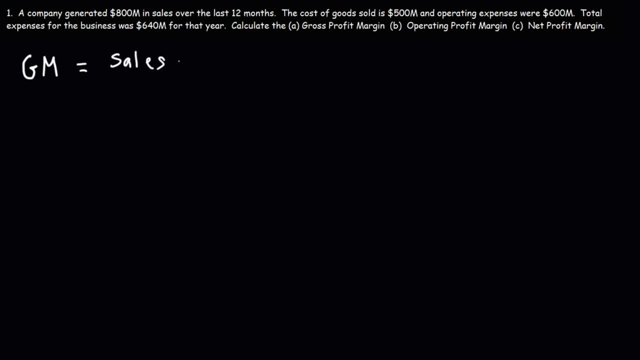 The gross margin is going to be the difference between the sales and the costs of goods sold, which we can abbreviate that as COGS, And all of that is going to be divided by the sales times, 100%. So the sales in this example is 800 million. The cost of goods sold is 500 million. 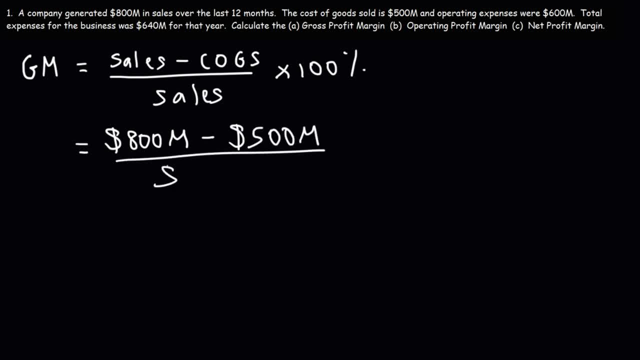 And we're going to divide that by 800 million and then multiply by 100%. So 800 minus 500, that gives us a gross margin of 300 million. But we want to get the gross margin as a percentage, So we need to divide it by the sales. 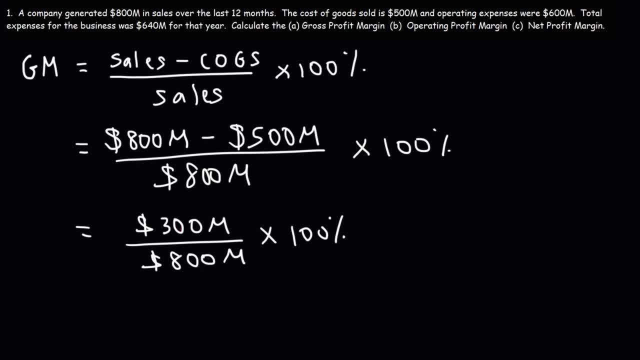 So 300 million divided by 800 million, if you cancel the two zeros and the M, it's going to be 3 over 8.. So 3 divided by 8, times 100, that gives us a percentage of 37.5%. 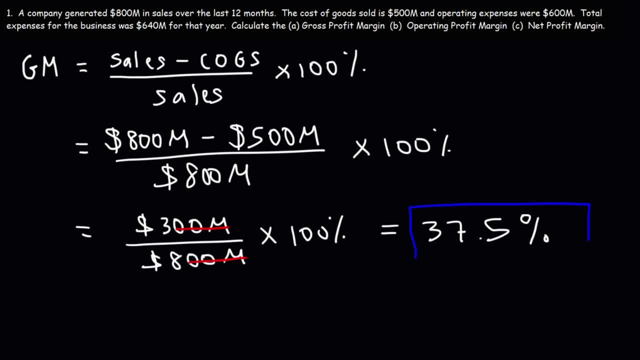 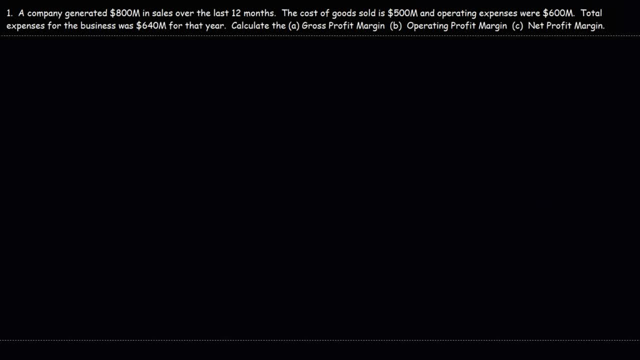 So that's how we can calculate the gross profit margin as a percentage. Now let's move on to part B: Calculate the operating profit margin. The operating margin is going to be the operating income divided by the sales times: 100%. Now, the operating income is the difference between the sales and the operating expenses. 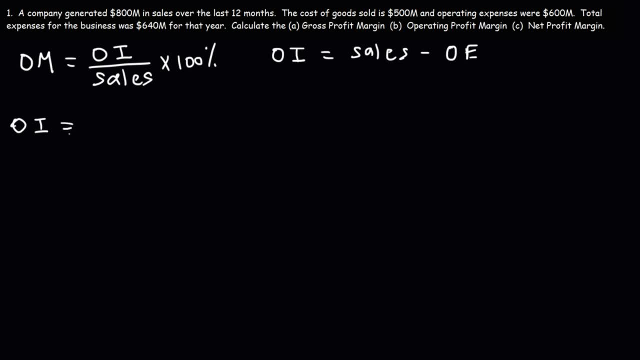 which I'm going to write as OE. So let's go ahead and calculate that first. So the company has 800 million in annual sales and the operating expenses for that year were 600 million. So that leaves behind an operating income of 800 million and the operating expenses for that year were 600 million. 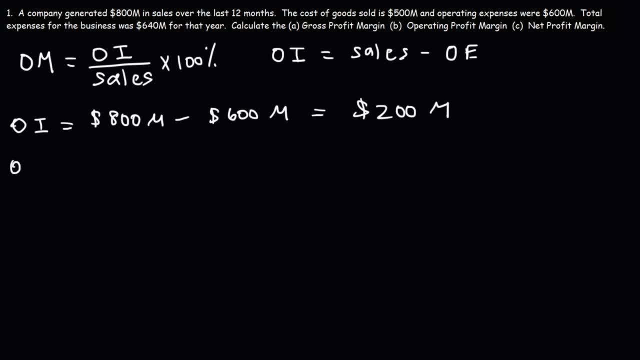 So that leaves behind an operating income of 200 million. So now to calculate the operating margin: it's going to be the operating income of 200 million divided by the sales of 800 million, and then times 100%. So this is going to be 2 divided by 8, times 100. 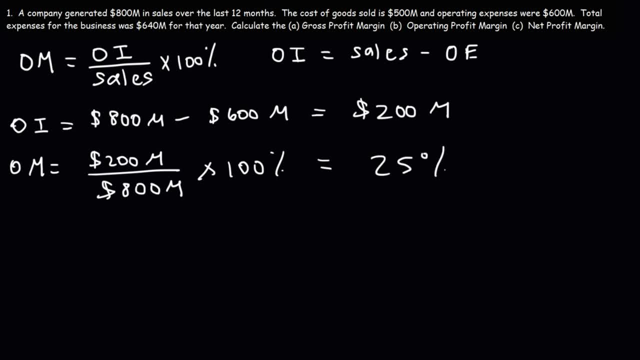 And so the operating margin as a percentage for this example is 25%. Now let's calculate the net profit margin. So that's going to be the revenue or the sales minus the total expenses which we could write as TE. 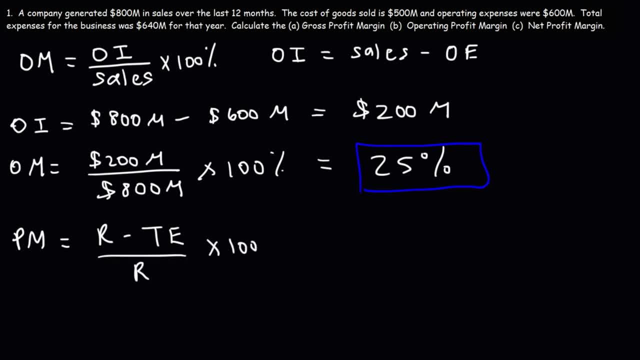 divided by the sales or the revenue. So the company had 800 million in revenue or annual sales, Total expenses were 640 million. So if we subtract 800 million by 640 million, that gives us a net income of 160 million over 800 million. 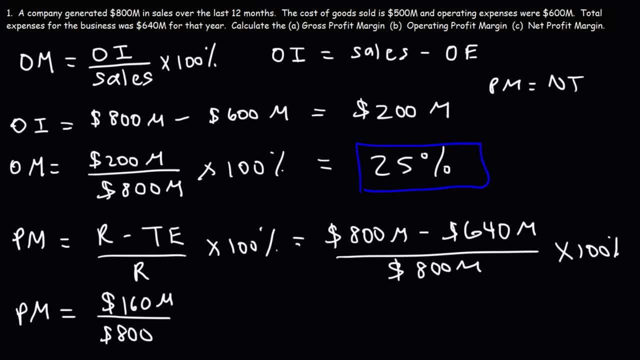 Keep in mind, the profit margin is the net income over the sales times, 100%. That's another way in which you could represent the formula, So I'm showing you different ways in which you might see it presented to you. So 160 divided by 800.. 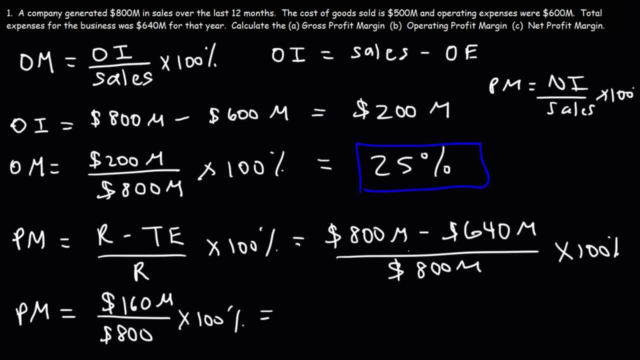 That's 0.2 times 100%. So this company has a profit margin, or a net profit margin of 20%. So now you know how to calculate the gross margin, the operating margin and the profit margin. Now let's move on to our next example. 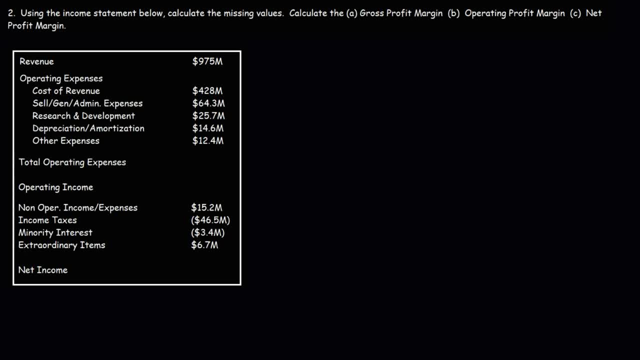 Using the income statement below, calculate the missing values And then calculate the gross profit margin, the operating profit margin and the net profit margin. So feel free to pause the video if you want to work on this example. So the missing values that we're missing are the total operating expenses, the operating income and, finally, the net income. 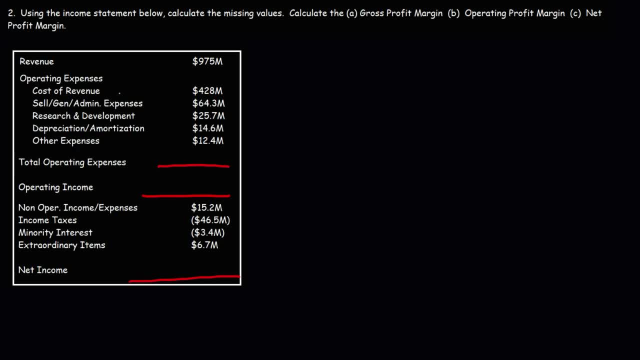 So let's start with this one: the total operating expenses. So here are all of the operating expenses. So we need to find a sum of those values. So it's going to be $428,000,000 plus $64.3,000,000, plus $25.7,000,000, plus $14.6,000,000 plus $12.4,000,000.. 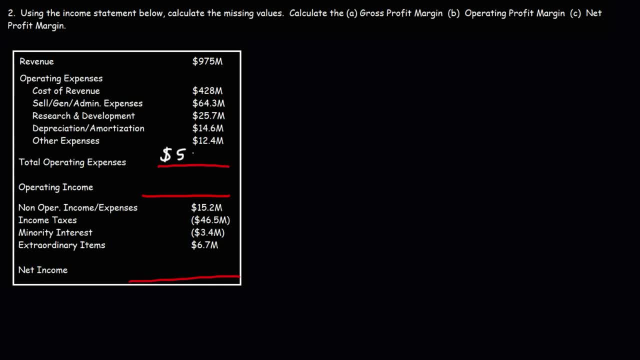 So the total operating expenses are $545,000,000.. Now we need to calculate the operating income. The operating income is the difference between the revenue and the total operating expenses. So we have a revenue of $975,000,000, and the total operating expenses are $545,000,000. 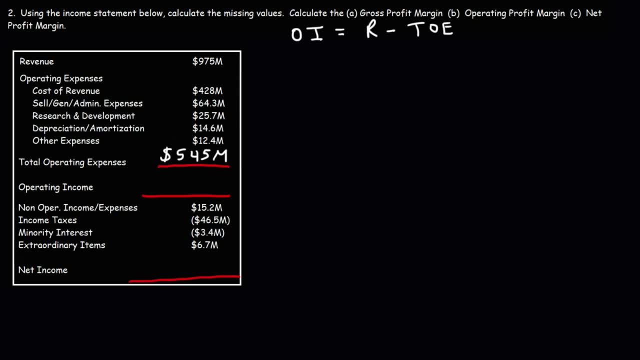 So let's subtract those two numbers: $975,000,000 minus $545,000,000.. So that's going to give us an operating income of $430,000,000.. Now the last thing we need to do is calculate the net income. 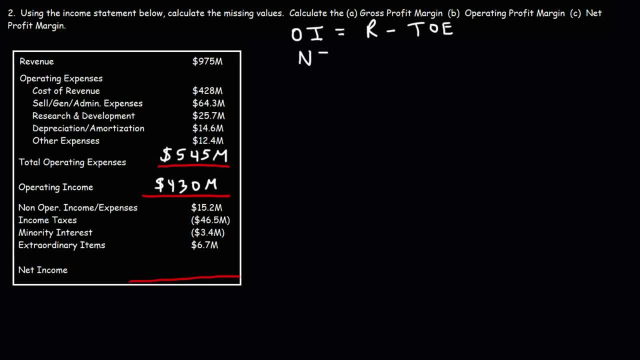 So the net income is going to be The revenue minus all of the expenses, or the total expenses. So it's going to be $975,000,000 minus all of the operating expenses, which is $545,000,000.. That gives us the operating income. 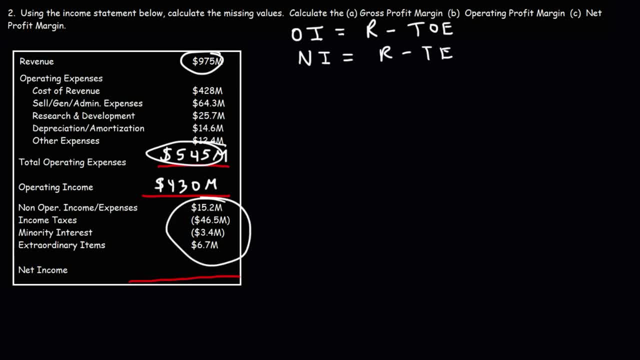 And then we need to take all these numbers into account. Now we need to determine which of these numbers are positive and which ones are negative. Income should be added, Expenses should be subtracted. So the $15.2,000,000 is that. 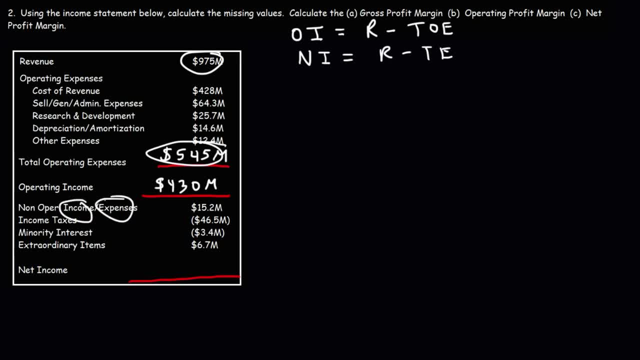 Positive or negative, because it can be income or expenses. Now, typically when you see a number in parentheses, particularly with financial statements, that indicates a negative number And, of course, income taxes. that's negative, That's an expense. 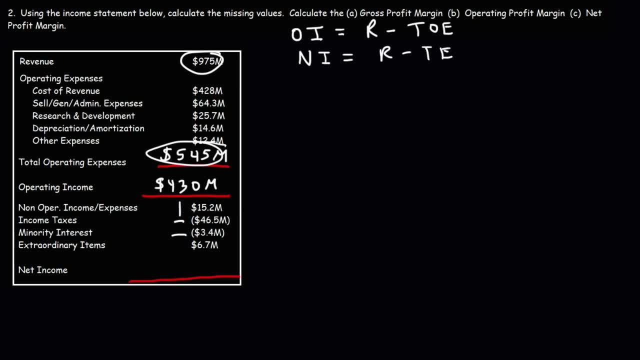 So we don't have parentheses here- which tells us that this number is positive, And the same is true for the extraordinary items. So right now, subtracting these two numbers give us an operating income of $430,000,000. And then we're going to add $15.2,000,000 to that. 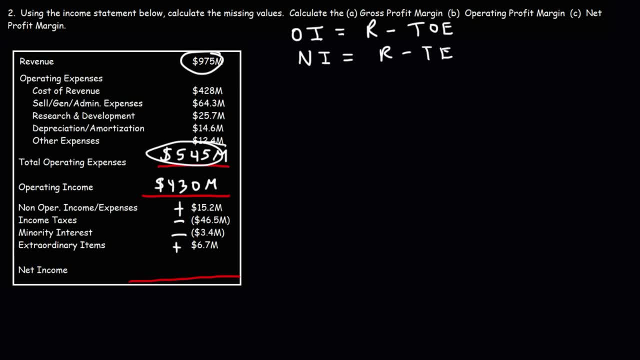 And then we're going to subtract by $46.5,000,000. And then subtract by $3.4,000,000. And then add by $6.7,000,000. So you should get $402,000,000.. 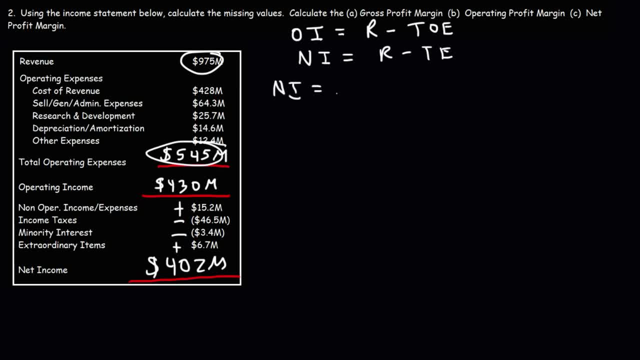 For those of you who missed that, here's the math. So we took the revenue of $975,000,000. Subtracted by the total operating expenses of $430,000,000. That gave us the operating income I mean minus $545,000,000. 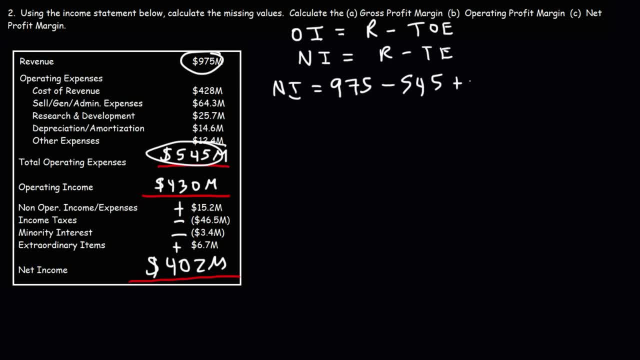 That gave us an operating income of $430,000,000.. And then we added $15.2,000,000, minus $46.5,000,, minus $3.4,000,000, and then plus $6.7,000,000.. 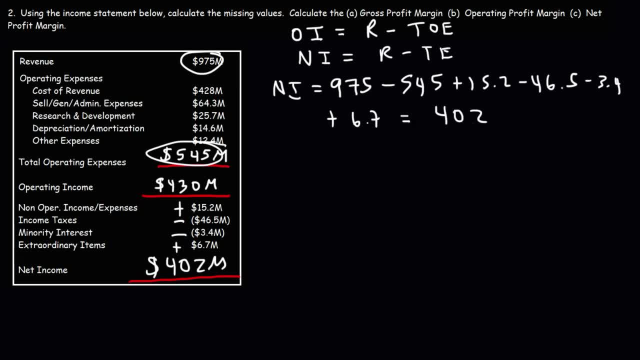 So that should give you $402,000,000.. Now let's start with Part A. Let's calculate the gross profit margin. So recall that the gross margin is going to be the difference between the sales and the cost of goods sold. 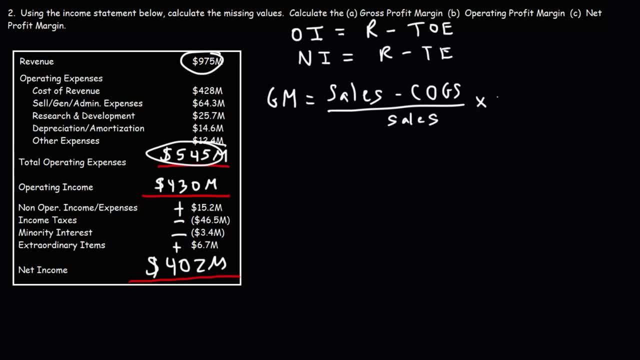 And then divided by the sales times, 100%. So the sales or the revenue is $975,000,000.. The cost of goods sold, in this case that would be $975,000,000.. The cost of revenue: that's $428,000,000, divided by the sales times 100%. 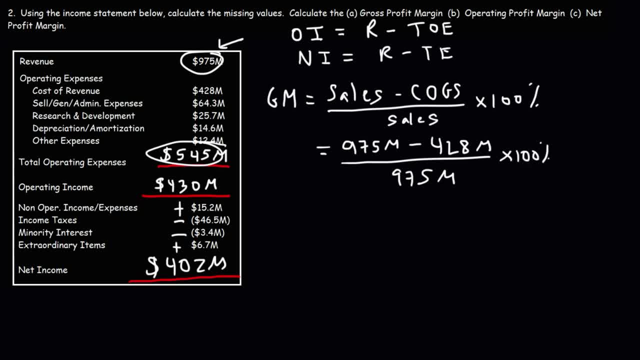 So $975,000,000, minus $428,000,000,, that's $547,000,000.. $547,000,000, divided by $975,000, is $0.561,000.. So, times 100%, this gives us a gross margin of 56.1%. 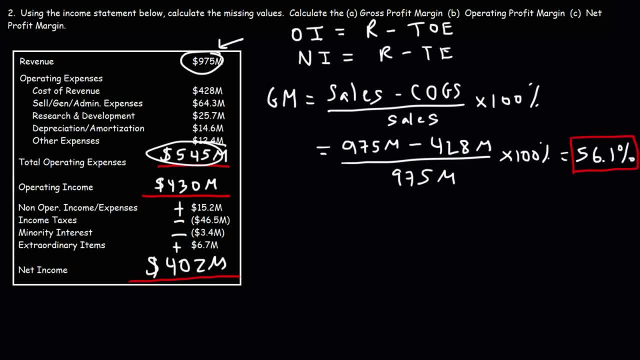 So that's the answer for Part A. Now let's move on to Part B. Let's calculate the operating margin. So the operating margin is going to be the operating income divided by the sales times, 100%. So we can see that the operating income is $430,000,000. 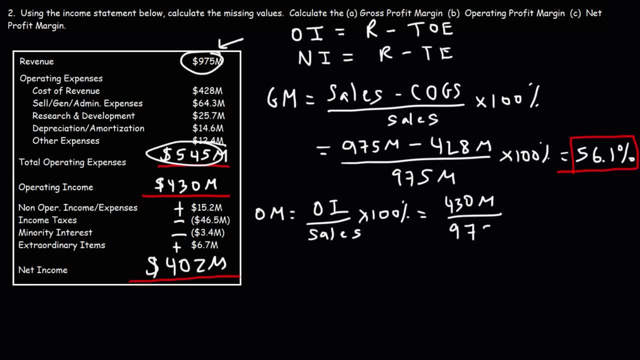 The sales or the revenue is $975,000,000.. So that's going to be the net margin divided by the sales times 100%. So it's Furlong's själva per cent. So $430,000,000, minus $ instantly.